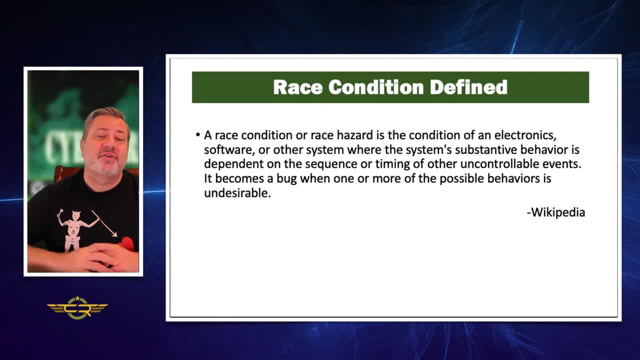 to first define what a race condition is. So this is a definition from our friends at Wikipedia. A race condition or race hazard is the condition of an electronics software or other system where the system's substantive behavior is dependent on the sequence or timing of other uncontrollable 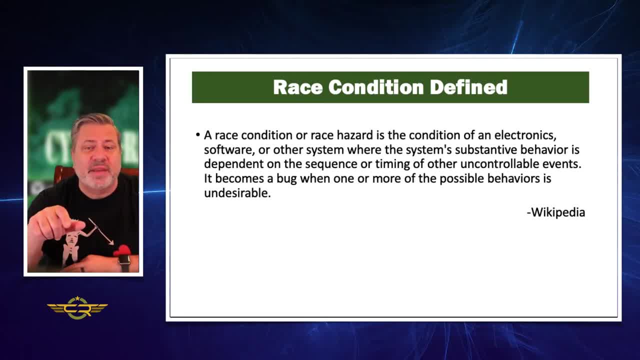 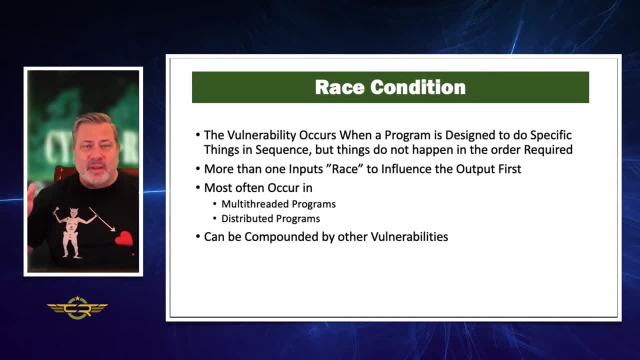 events. It becomes a bug when one or more of the possible behaviors is undesirable. So really, we're having something happen that should happen in sequence and the program has defined the sequence, but somehow it's not. So we're having something happen in sequence and 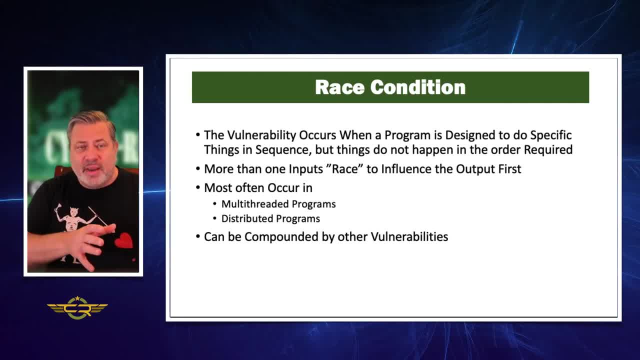 somehow, when they built the program, when they built the software, that sequence isn't always followed and the input is not always handled in the order that the programmer wanted it handled in. So it's a bug because it has to be fixed. It's really hard to find these, So they're normally 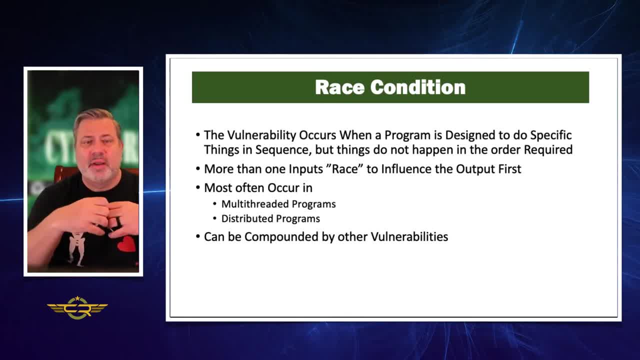 found in the wild when people start using the software, and that's really why we have to have strong testing, user acceptance testing, component testing and security testing Before a project goes live in into an actual program that we release to the wild. So this 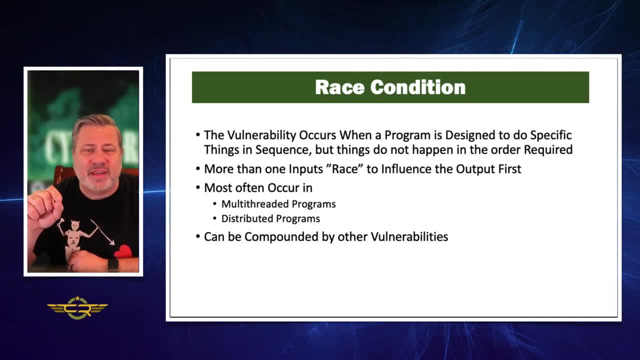 vulnerability occurs when a program is designed to do a specific thing in sequence but things do not happen in the order required, right? So more than one inputs race to out, more than one input race to influence the output first. So we want things to happen one, two, three, four, five and 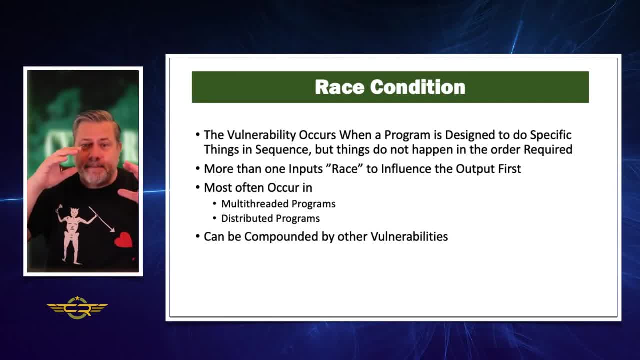 somehow they happen one, two, three, four, five. and somehow they happen one, two, three, four, five, three, two, one or whatever. They don't happen the way the programmer wanted them to happen. And that's an issue, because if we're handling things like transactions of cash or the way 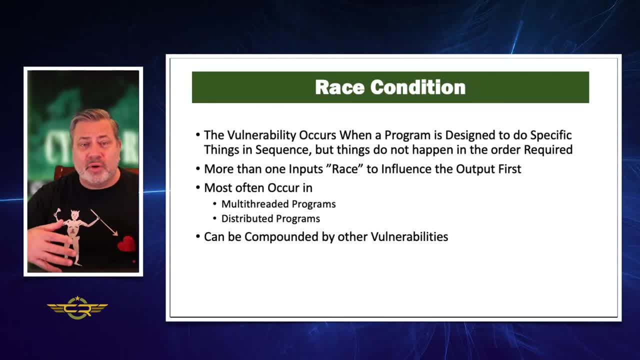 something needs to happen for the project to go forward or for the application to work correctly. inputs getting to the output in the wrong order could cause maybe somebody to have more or less money than they should have, or it could cause the system to crash altogether. This happens. 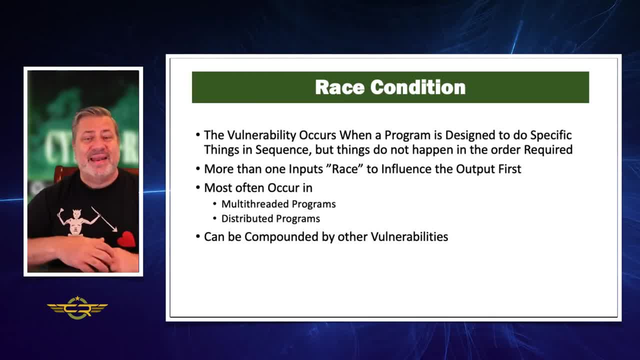 a lot of times. This happens a lot in multi-threaded programs or distributed programs, and it can be compounded by other vulnerabilities. So it's really the things we need to know about. race conditions is more than one input. is racing to influence the output first? Things are not happening in the sequence that the 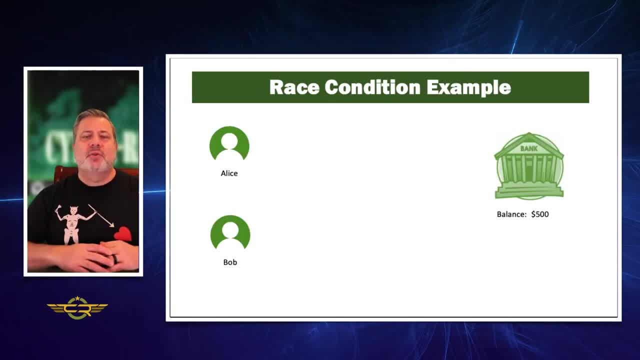 programmer wanted them to happen. So if we look at this in a very, very simple demonstration of what it could look like in the real world- not in a program, but in a real world- we're going to say: this was the real world. We want things to happen in a specific sequence. So Alice knows that. 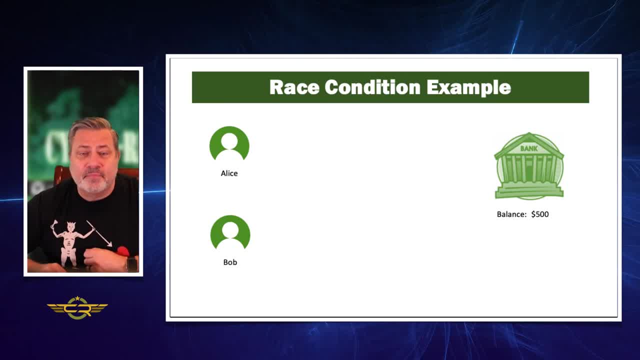 her balance in the bank is $500. So she deposits $1,000.. That should make her balance go up by $1,000 to $1,500. But about the same time Bob cashes a check from Alice in the amount of $700, right. 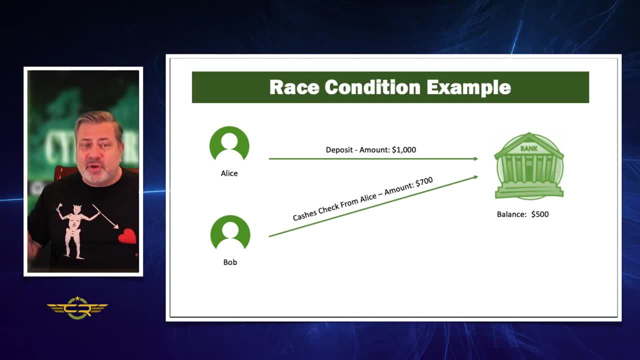 So now we've got two transactions or two, two input values going towards the bank. Now, if the bank does not sequence things correctly- right, even though that deposit may get there a bit earlier, if it's not sequenced correctly the way it processes through the bank, Alice's balance may be actually negative $200 because 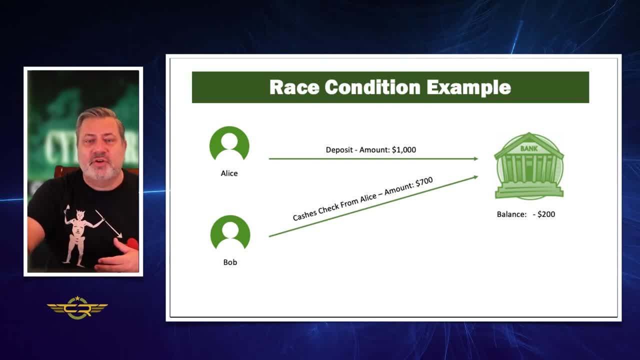 Bob's check may get there first and she only has that $500 balance $700 out. that leaves her a negative $200.. Even though she had a $1,000 deposit coming in Now, more than likely the deposit would be processed next. 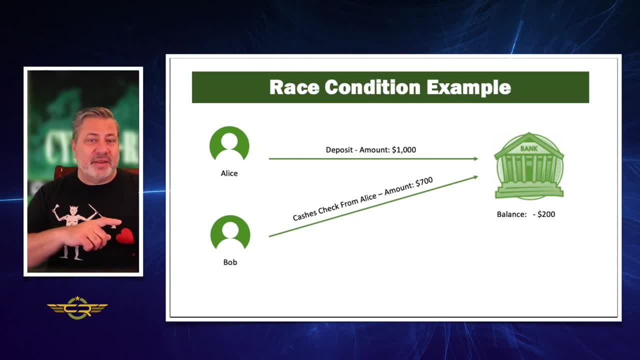 and that would bring her balance back up. But there may be things like overdraft charges or the check may even get returned to Bob. So this is a very simple example of a race condition. So there's two inputs coming in In this case. the first input is the deposit of $1,000.. The second 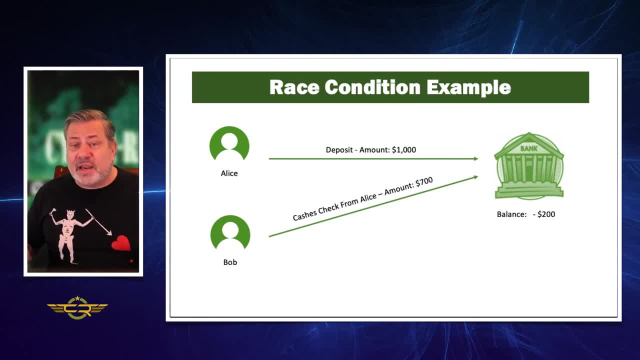 input. is the withdraw a $700 from the check That's going to impact the balance of $1,000.. That's going to impact the output or her balance. So we really want to watch these things, We want to look out for them in our programming And if we're the security professional, that's there. 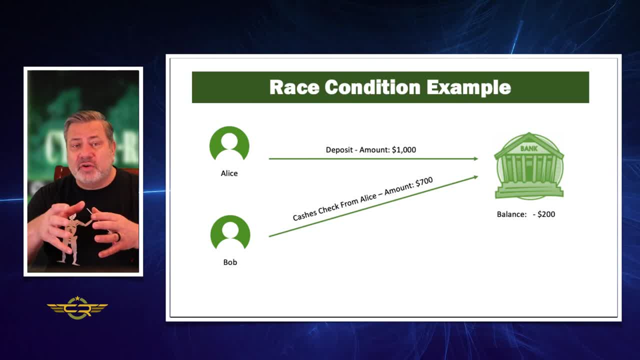 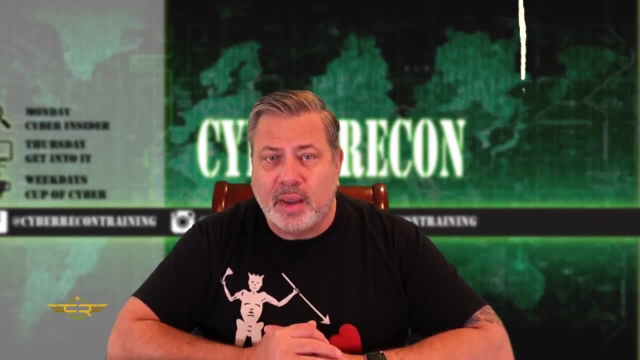 to make sure that the programs are secure. we have to look for these things either through manual code review or automated code review. So, as always, I'm Jim with Cyber Recon here, helping you get better at your security career, hopefully getting you. 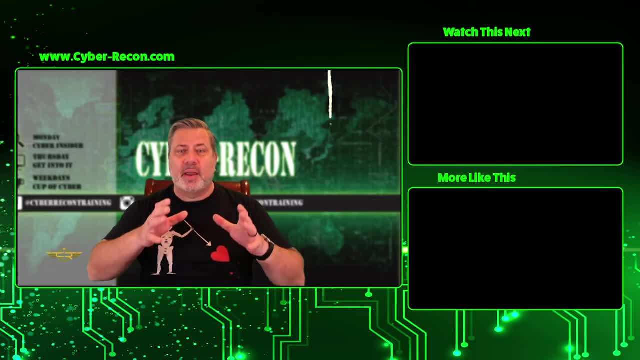 moved up the security ladder and to bigger and better things, As always. we'd love you to subscribe like comment, hit the bell to be notified and we will see you next time. Be careful out there.